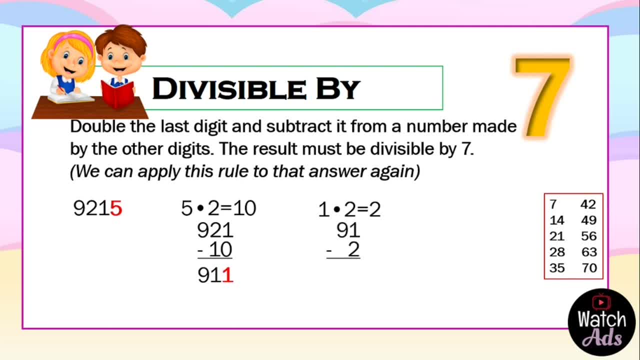 91.. 91 less 2 is equal to 89.. Next is we double again The last digit, that is 9,, gives 18.. Then subtract it from 8.. 8 plus 18 is equal to. Well, if you're in middle school or high school, you already know how to double. 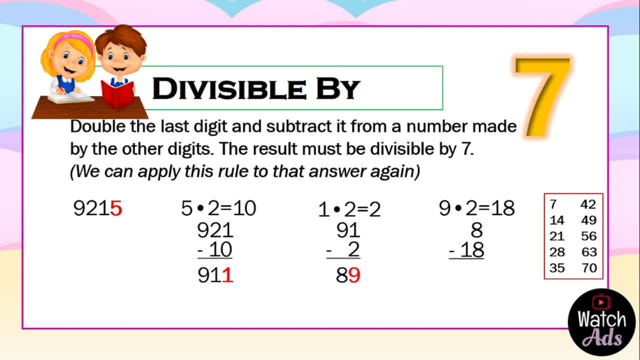 integers the rules of signed numbers, which means that you can answer this. but don't worry, if you're still in grade 4, and you don't know the rules of signed numbers, you just simply subtract 18 less 8. the answer is 10.. still, 10 is not divisible by 7, which means that 9215. 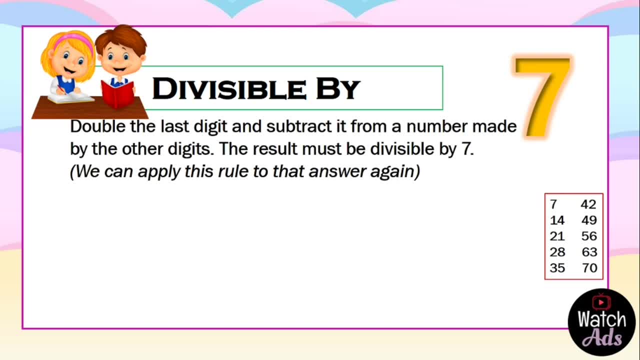 is not divisible by 7.. the example: 1093: we double the last digit, that is 3, it gives us 6.. we subtract 6 from 109, the answer is 103.. again, we double 3, it gives us 6.. we subtract 6 from 10. 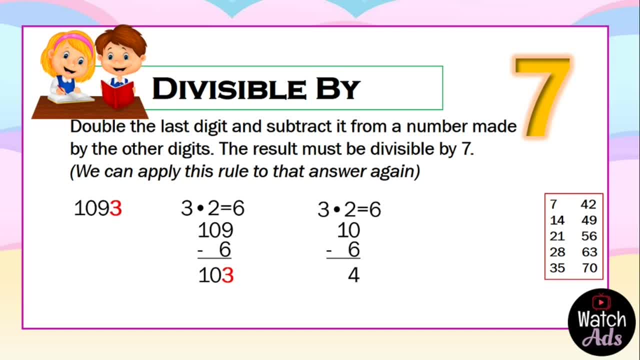 the answer is 4.. still, 4 is not divisible by 7, which means 1093 is not divisible by 7.. our last example is 5796.. we check the last digit, that is 6, and then we double it, which gives us 12.. subtract 12 from 579, the answer is 567.. next, the last digit is 7.. 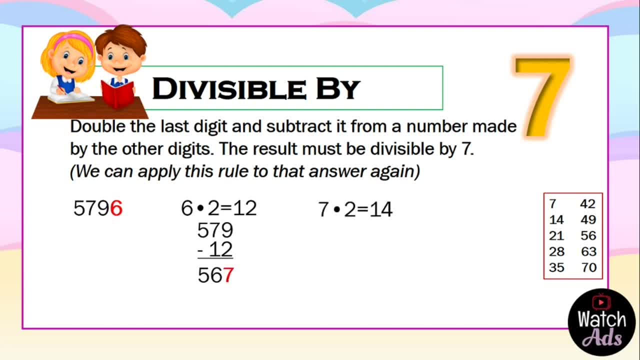 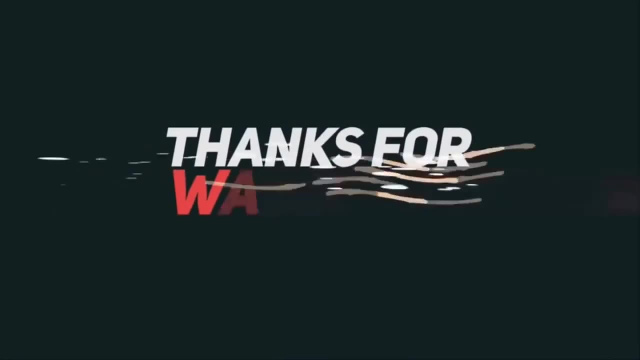 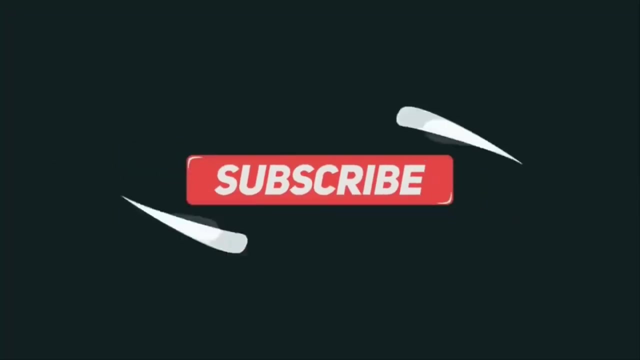 we double 7, it gives 14.. subtract 14 from 56.. the answer is 42.. now we know that 42 is divisible by 7, which means that 796 is divisible by 7..